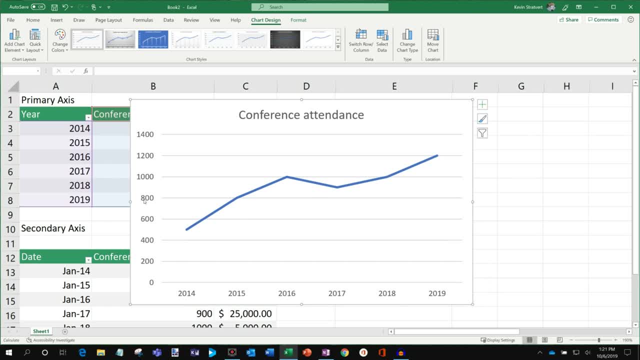 and here what you'll see is, I have my line chart, I have the number of attendees on the y-axis or the vertical axis, and then here I have the years on the horizontal axis. and then here I have the years on the horizontal axis. 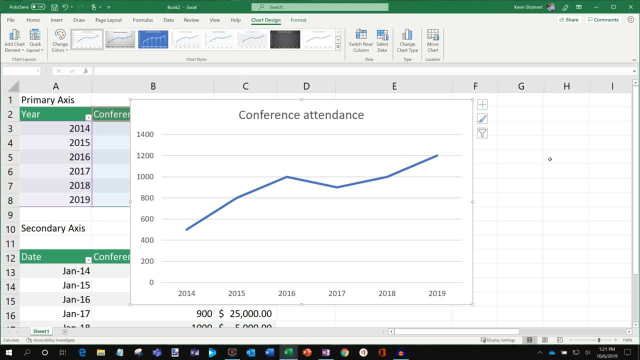 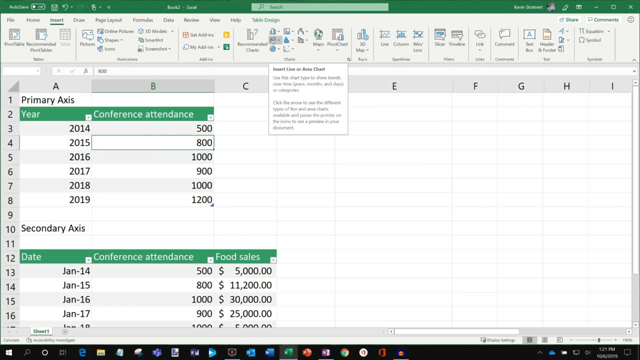 So another way that we could also do this. I'm going to go ahead and get rid of this for now. I could go back to insert, and here you'll see that I also have an option to insert a line or area chart. So I have all these different options here, but I'm going to go ahead and click on this. 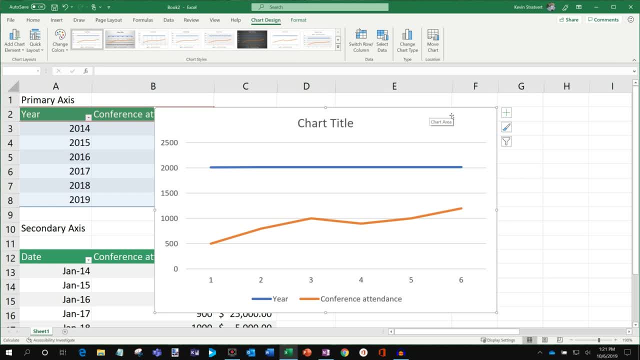 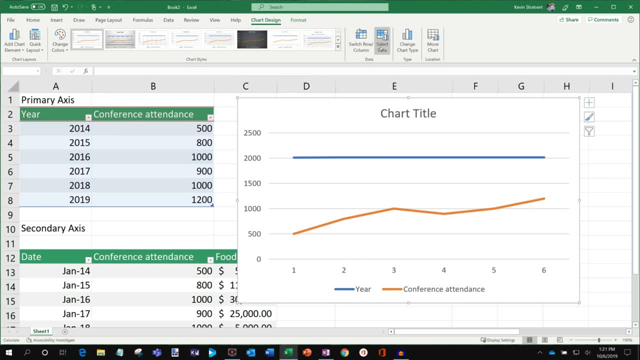 line one When I insert this. unfortunately, it's not quite as easy as the recommended chart, but let me show you how I can get this chart to work with my data that I have here. So what I'm going to do is I'm going to click on this option that says select data on the top bar. 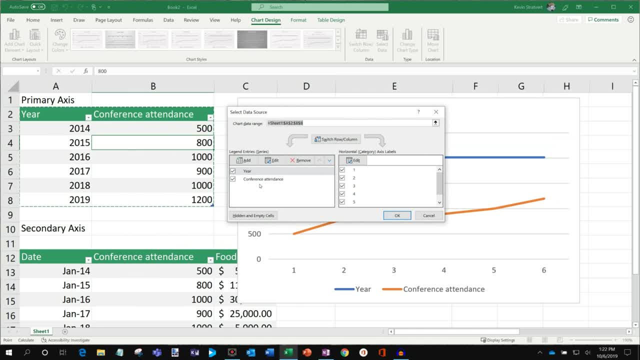 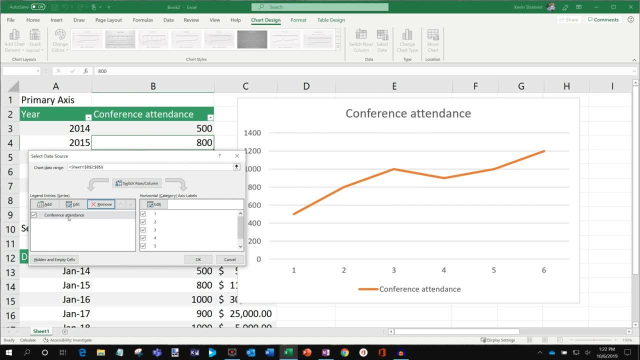 and what you'll notice here is: these are my different line charts. Well, I don't want to chart out the year, because that's simply going to advance throughout the year, so I'm going to get rid of that. and so I want to map out the conference attendance over time, So I'm going 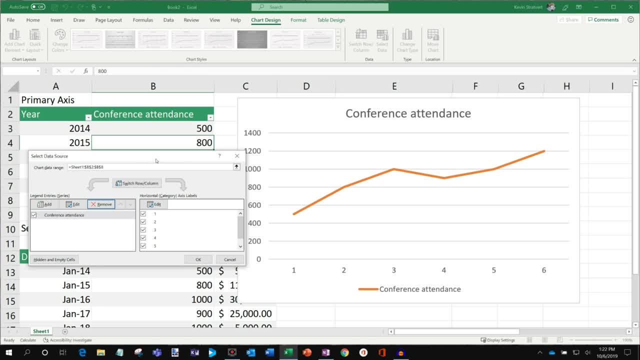 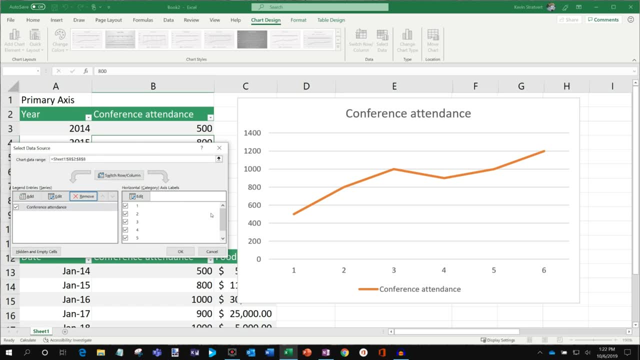 to leave that here as a legend, entries or series. Now what you'll see is here it says the horizontal axis. so this is the horizontal one. Right now it just goes from one to six, but I want that to be the year. So what I'm going to do is I'm going to click on edit. 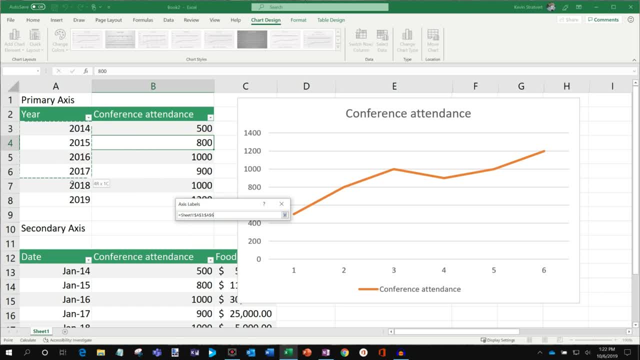 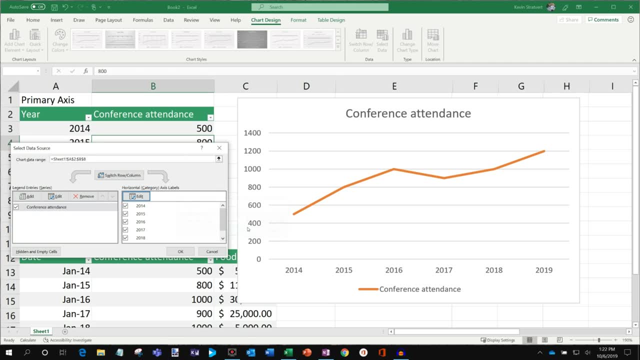 and what I want the range to be is. instead, I want that to be the year here, So I'm going to go ahead and highlight the year, and then you'll notice that it appears immediately down here in my chart. So I'm going to go ahead and click on okay. and this all looks good, So I'm going to click on okay. 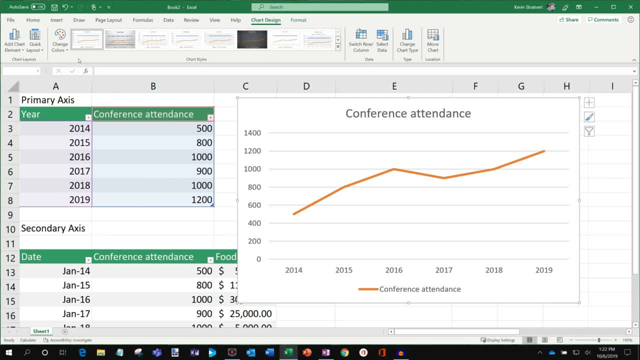 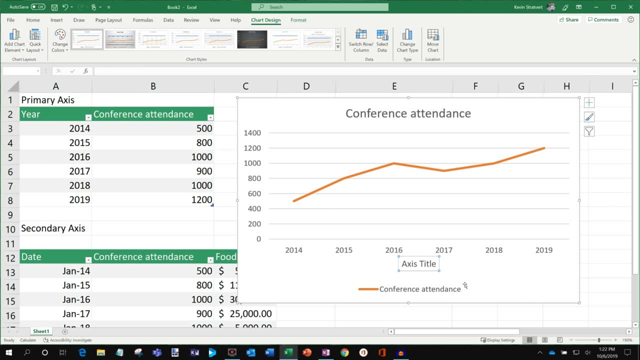 and so here you see the attendance by year. Now what I could also do is, if I click on add chart element, I could add labels for these. So let me add the primary horizontal label first. So I'm going to click here and what I could do is here I could just say this is the year, and I could 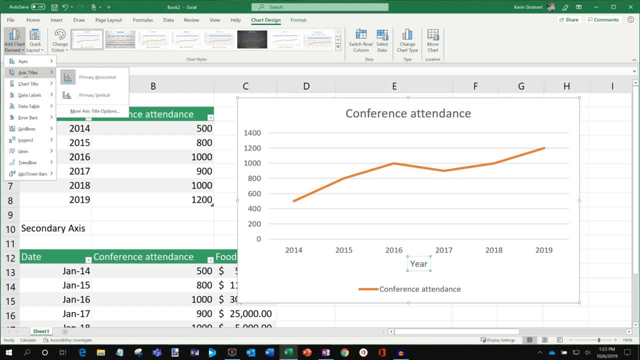 also add another axis title. So I'll go back to the add chart element, axis titles and I'll add a vertical title in here and maybe I'll just call this attendees And I could also get rid of this element down here, since it's pretty clear, since there's just one thing that I'm charting out. 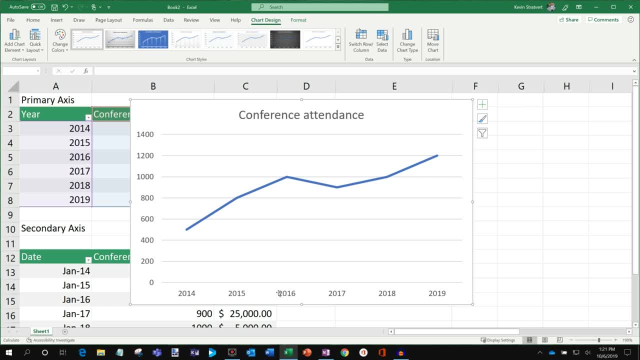 on the y-axis or the vertical axis, And then here I have the years on the horizontal line chart, and then here you'll see what's recommended. So I'll see a lot more Run this way. So we hit set. come back to Braille Button. check those links. everything looks spot-true. 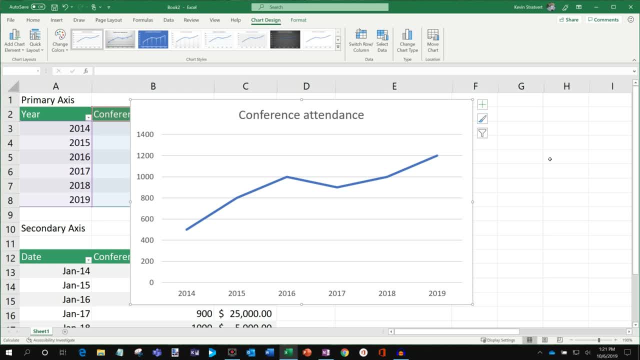 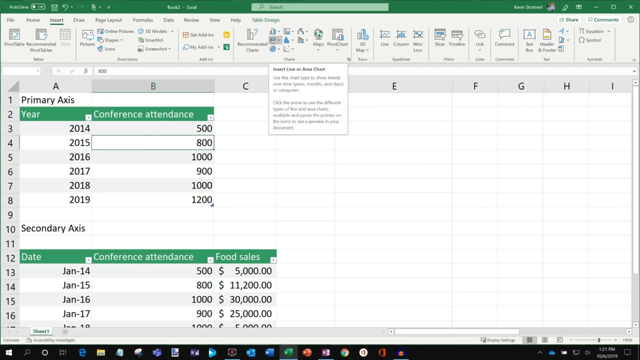 axis or the X axis. So another way that we could also do this. I'm going to go ahead and get rid of this for now. I could go back to insert, and here you'll see that I also have an option to insert a line or area chart. 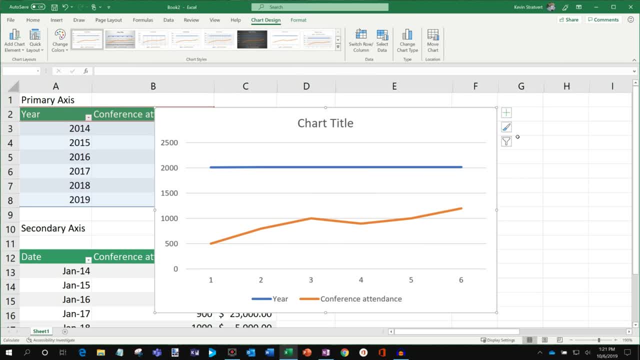 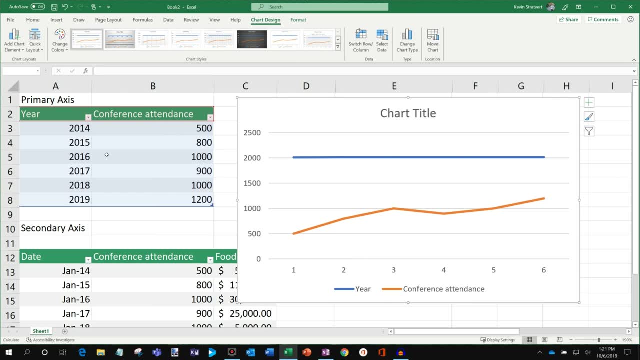 So I have all these different options here, but I'm going to go ahead and click on this line one When I insert this. unfortunately, it's not quite as easy as the recommended chart, But let me show you how I can get this chart to work with my data that I have here. 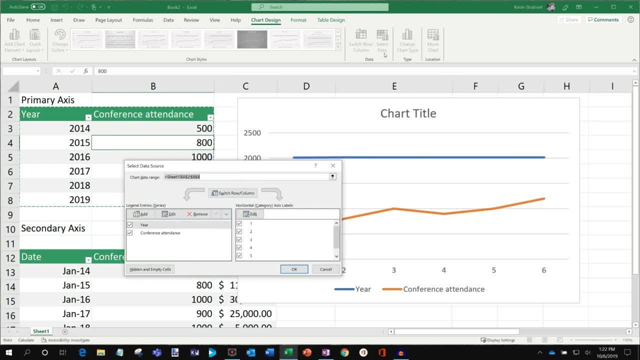 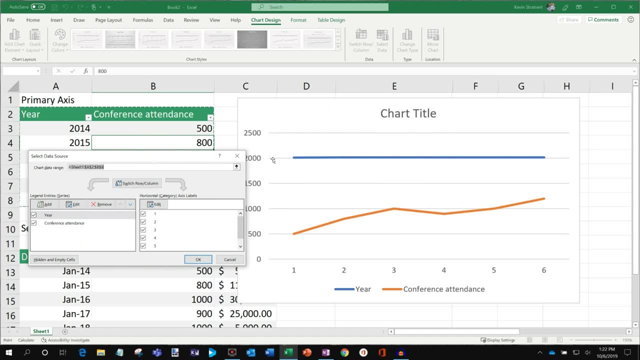 So what I'm going to do is I'm going to click on this option that says select data on the top bar, And what you'll notice here is these are my different line charts. Well, I don't want to chart out the year, because that's simply going to advance throughout. 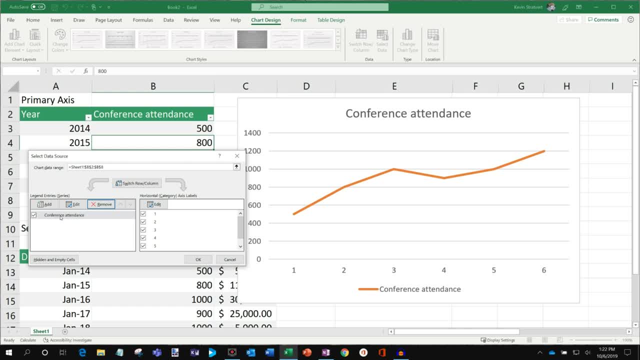 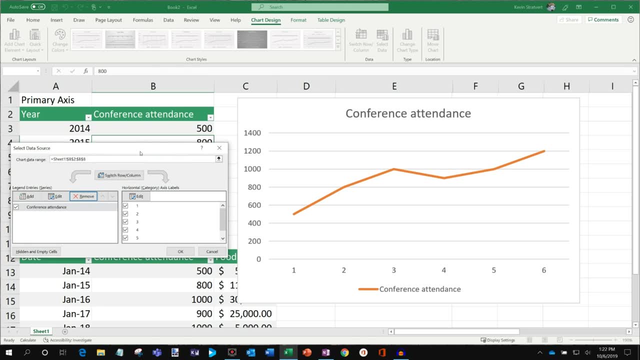 the year. So I'm going to get rid of that, And so I want to map out the conference attendance over time. So I'm going to leave that here as a legend entries or series. Now what you'll see is here. it says the horizontal axis. 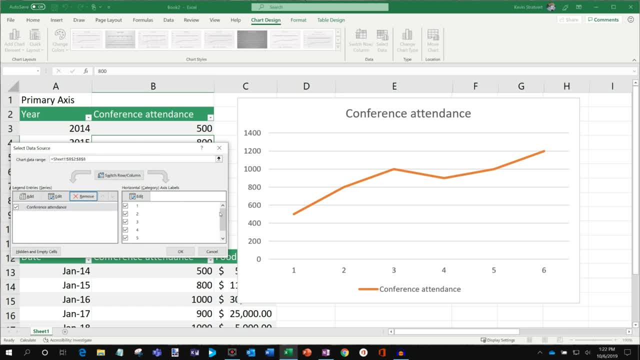 So this is the horizontal one. Right now it just goes from one to six, but I want that to be the year. So what I'm going to do is I'm going to click on edit, And what I want the range to be is instead: I want that to be the year here. 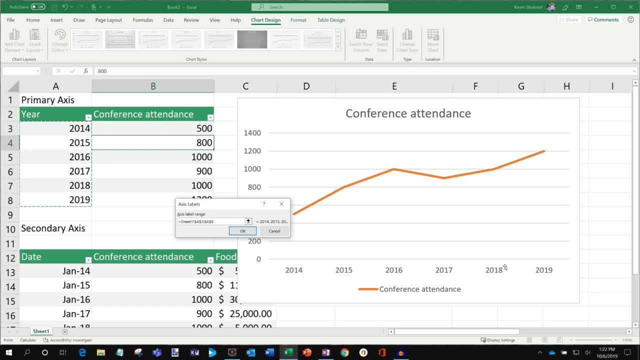 So I'm going to go ahead and highlight the year And then you'll notice that it appears immediately down here in my chart. So I'm going to go ahead and click on OK. And this all looks good, So I'm going to click on OK. 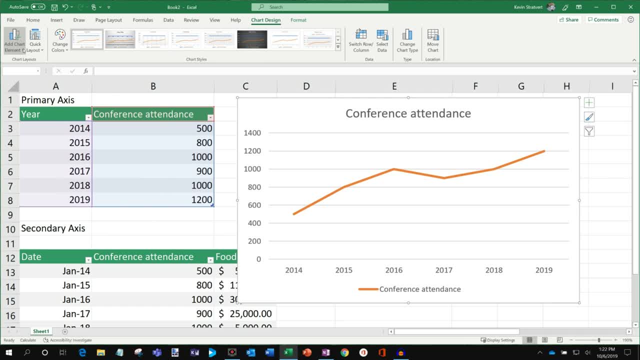 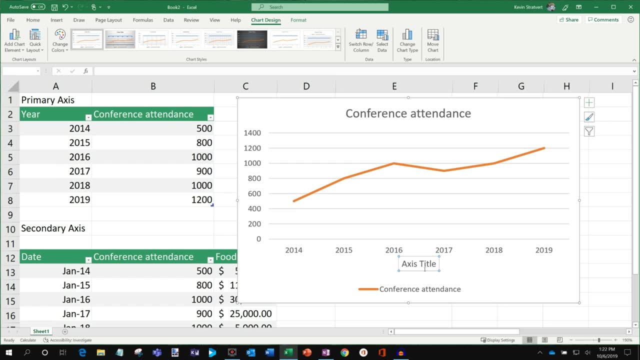 And so here you see the attendance by year. Now what I could also do is, if I click on add chart element, I could add labels for these. So let me add the primary horizontal label first. So I'm going to click here And what I could do is here I could just say: this is the year. 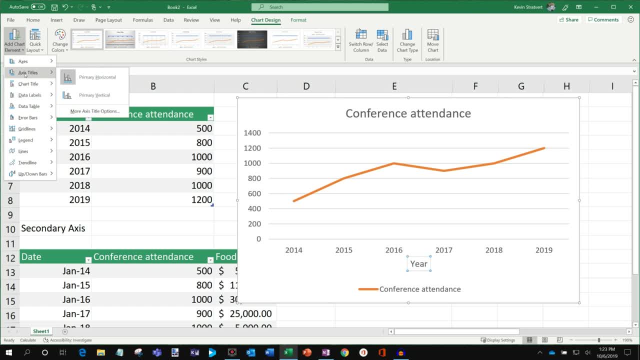 And I could also add a number. I could add another axis title. So I'll go back to the add chart element axis titles and I'll add a vertical title in here And maybe I'll just call this attendees And I could also get rid of this element down here, since it's pretty clear, since there's. 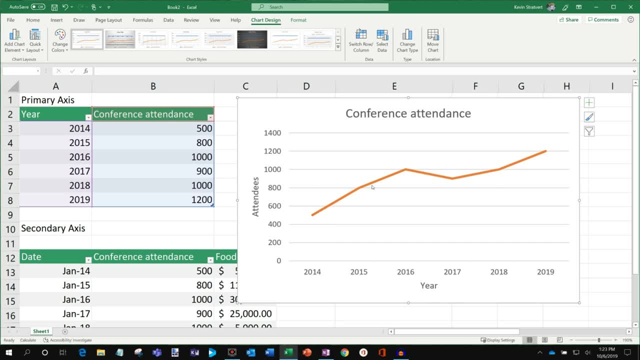 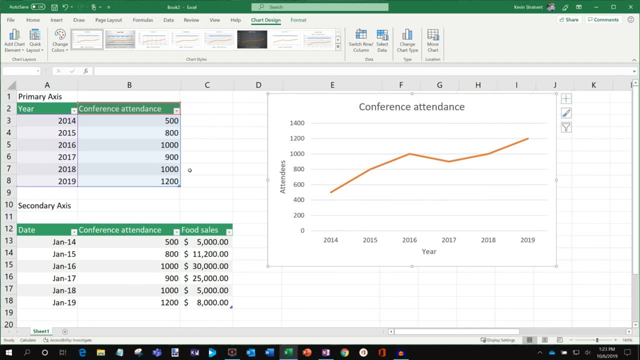 just one thing that I'm charting out. So here this is another way to create the same view, or to create a simple line chart. Now, what I also wanted to show is how you can create a line chart if you have multiple pieces of information and you want two different axes of information. 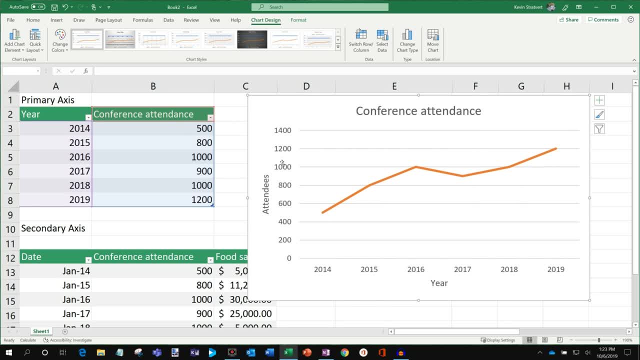 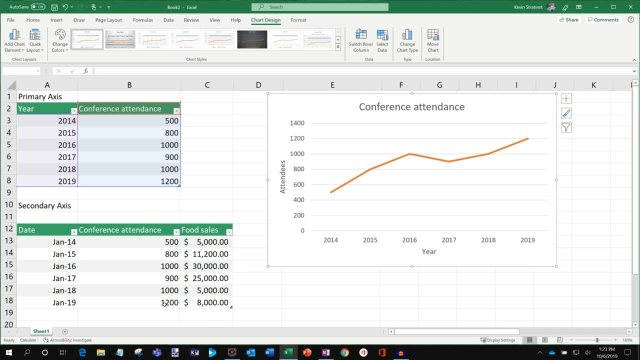 So here this is another way to create the same view or to create a simple line chart. Now, what I also wanted to show is how you can create a line chart if you have multiple pieces of information and you want two different axes of information. So here, once again, I have a set of data. It's the same data as above, where I have my 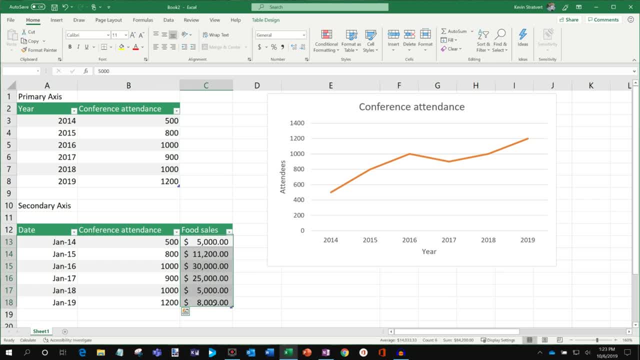 year, then I have my conference attendance, but now I also have food sales for those different years. So how do I visualize that? Well, what I'll do is I'll go back to insert, and what I'm going to do now is I'm going to click on recommended charts, and here you see a bunch of recommendations. 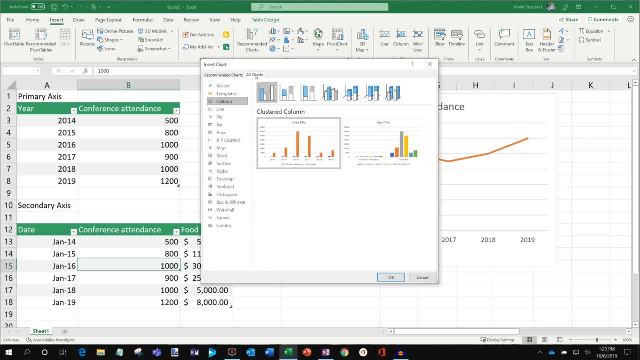 None of them are exactly what I want. So actually, I'm going to go ahead and click on all charts and now you see the full set of options I have, Because I have two different axes. this is what's going to look like, So I'm going to click on combo and here you'll see that there are two. 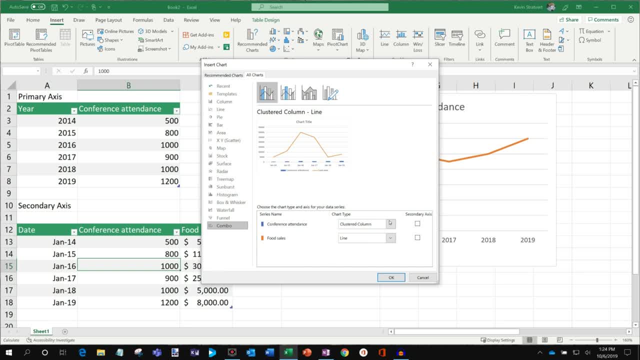 sets of information. I have my attendees and my food sales, So what I could do is for the conference attendance. maybe what I want to do is I could go with the column that looks good and then the line for the food sales looks good, But what I want to do is, rather than having them, 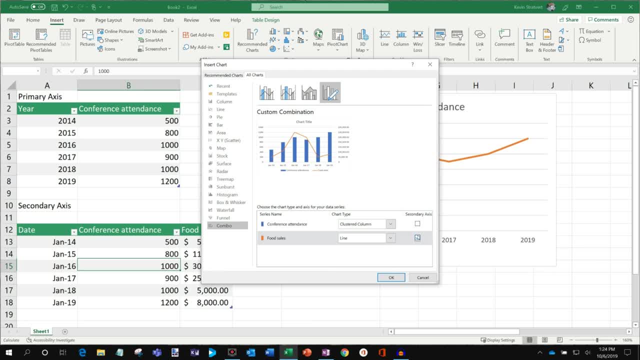 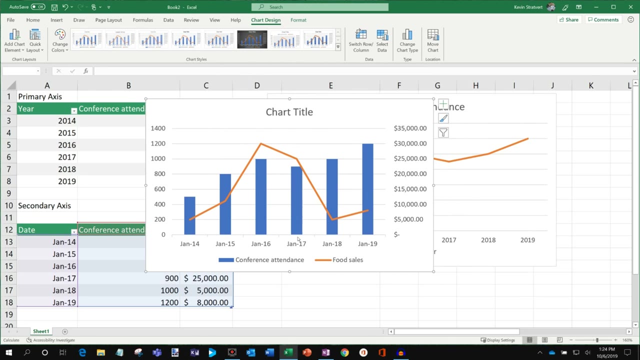 both go off the same axes. instead, I want to say: this is my secondary axes, And so now what you'll see is the conference attendance is on my primary axes right here, and then my secondary access is the food sales. So I'm going to go ahead and click on, okay, and now you'll see that it shows. 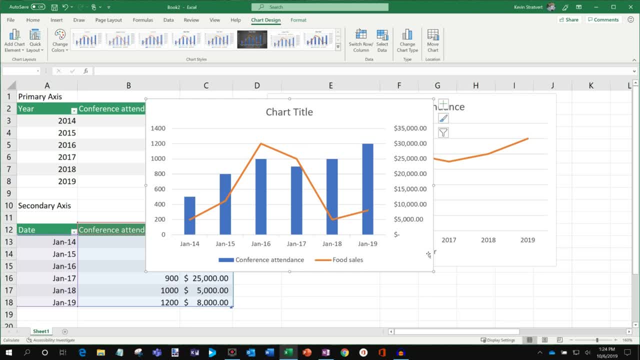 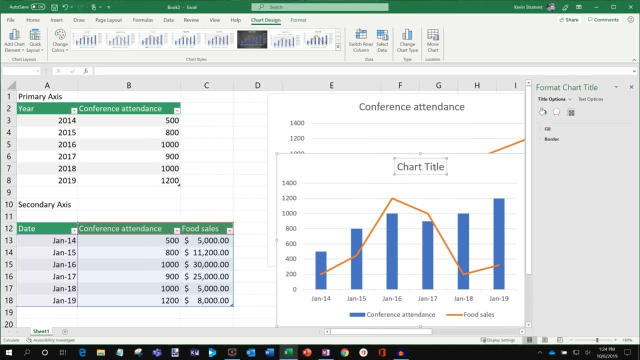 two sets of information, using this left-hand side and the right-hand side to display this combo information. So just another way to create a chart. and then maybe what I'd want to do is I could retitle this, and it could be conference attendance and food sales. So there I'm able to. 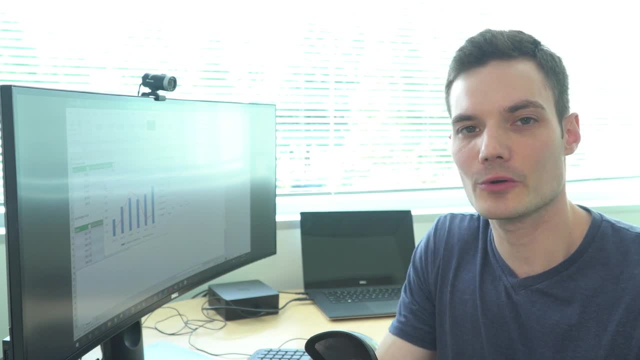 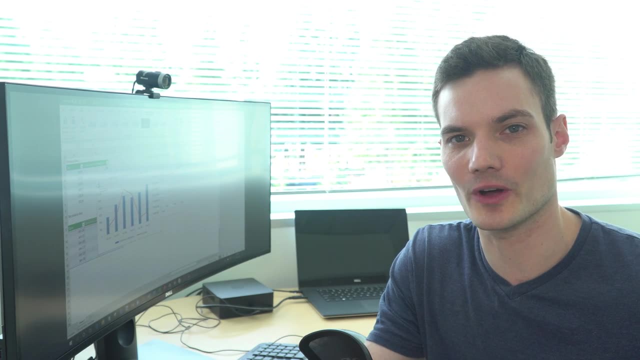 chart out two sets of information. So that was just a really quick tutorial on how you could create a really simple line chart in Microsoft Excel, whether you're just showing one set of information or whether you're using two sets of axes- the primary and the secondary. But that's. 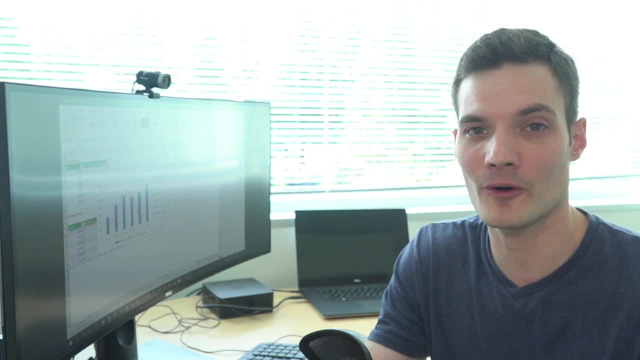 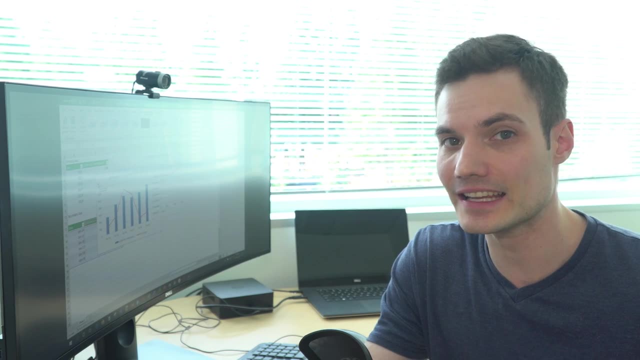 really as simple as it is. Hopefully you found this tutorial helpful. If you did, please give a thumbs up. If you want to see future videos like this, hit that subscribe button, And if you have any other ideas or anything else that you want to learn about, leave a comment down below. I read: 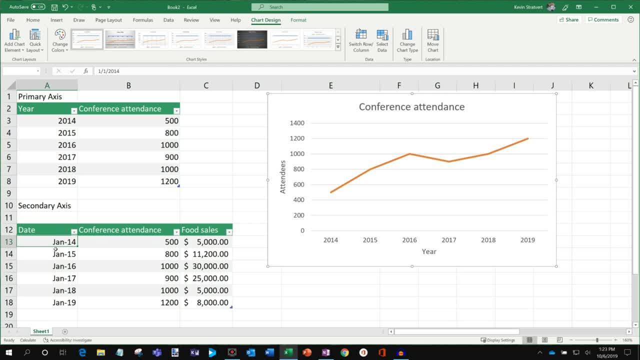 So here, once again, I have a set of data. It's the same data as above, where I have my year, then I have my conference attendance, but now I also have food sales for those different years. So how do I visualize that? Well, what I'll do is I'll go back to insert, and what I'm going to do now is I'm going. 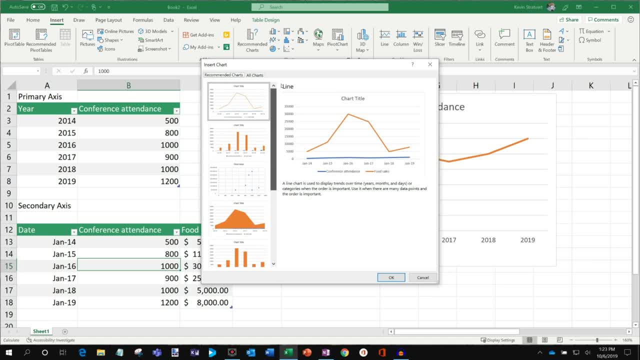 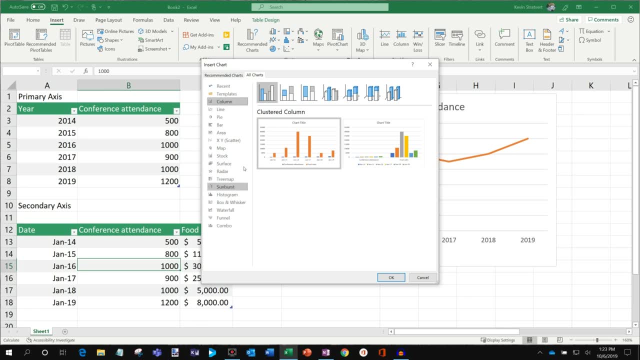 to click on recommended charts, And here you see a bunch of recommendations. None of them are exactly what I want, So actually, I'm going to go ahead and click on all charts, And now you see the full set of options I have, because I have two different axes. 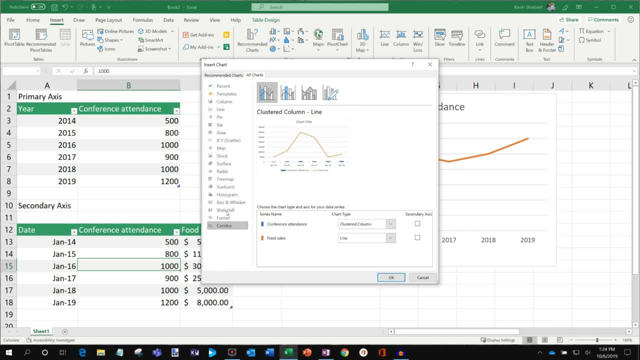 This is what's referred to as accommodations. So I'm going to click on combo charts, So I'm going to click on combo and here you'll see that there are two sets of information. I have my attendees and my food sales. So what I could do is for the conference attendance, maybe what I want to do is I could go with 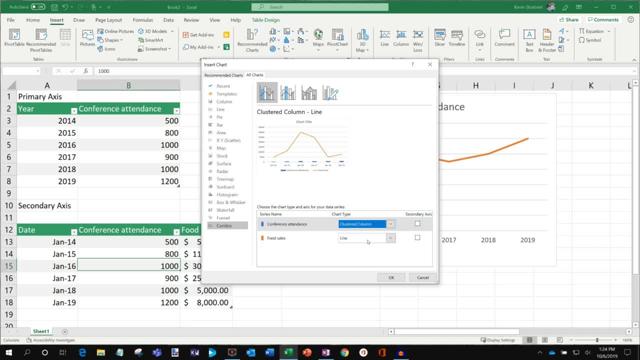 the column. That looks good, And then the line for the food sales looks good. But what I want to do is, rather than having them both go off the same axes, instead I want to say: this is my secondary axes, And so now what you'll see is the conference attendance is on my primary axes, right here. 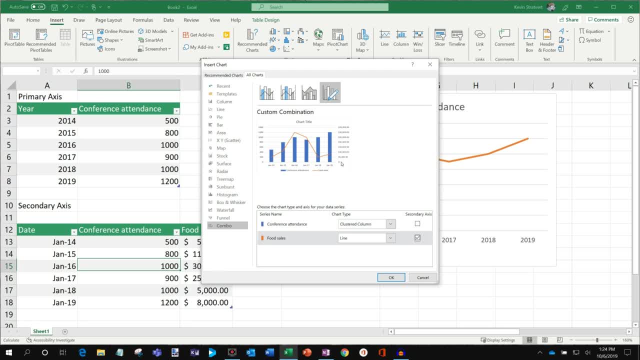 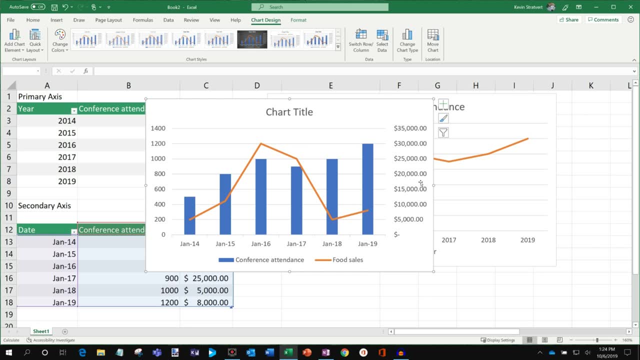 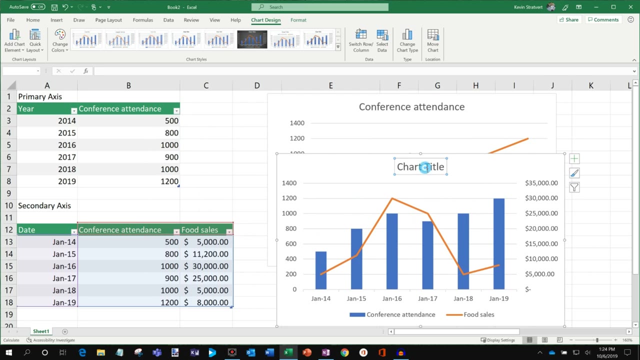 and then my secondary axes. So I'm going to go ahead and click on ok. Now you'll see that it shows two sets of information, using this left-hand side and the right-hand side to display this combo information. So there's another way to create a chart, and then maybe what I'd want to do is I could. 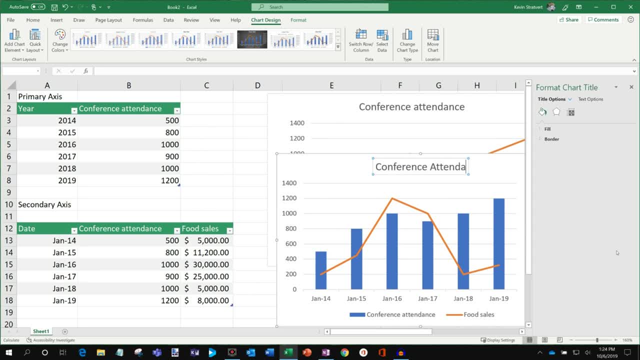 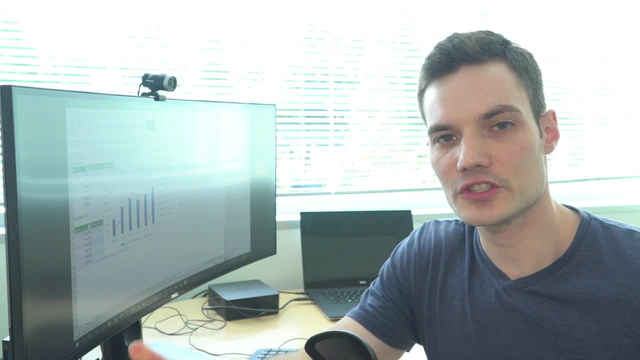 retitle this, and it could be conference attendance and food sales. So there I'm able to chart out two sets of information. So that was just a really quick tutorial. you could create a really simple line chart in Microsoft Excel, whether you're just showing, 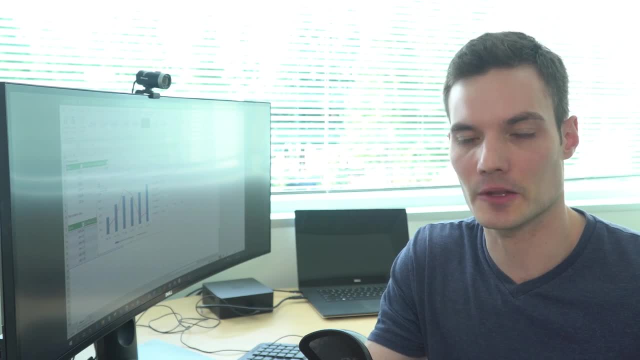 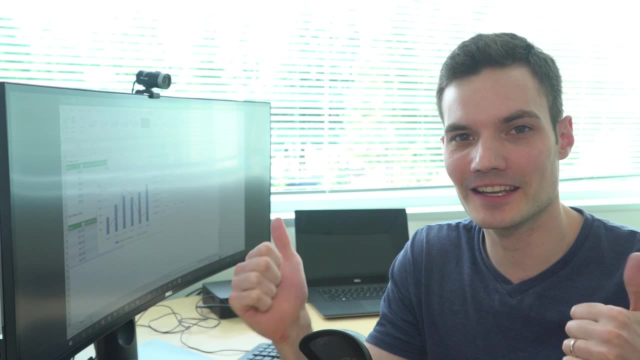 one set of information, or whether you're using two sets of axes, the primary and the secondary, But that's really as simple as it is. Hopefully you found this tutorial helpful. If you did, please give it a thumbs up. If you want to see future videos like this, hit that subscribe button. 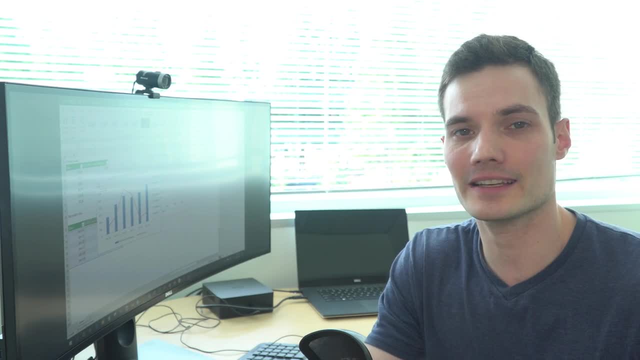 And if you have any other ideas or anything else that you want to learn about, leave a comment down below. I read all of them and I'll add it to my list of videos to create in the future. All right, Well, that's all I have for you today. I'll see you next time. Bye-bye.